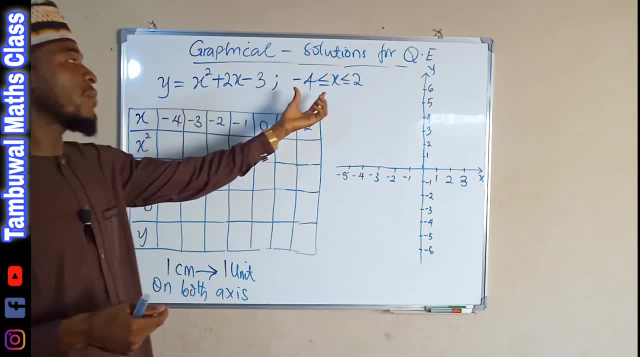 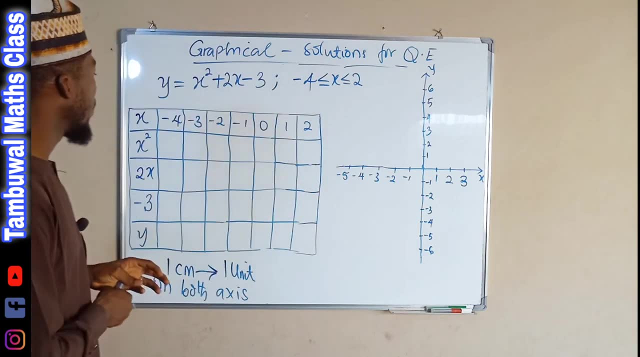 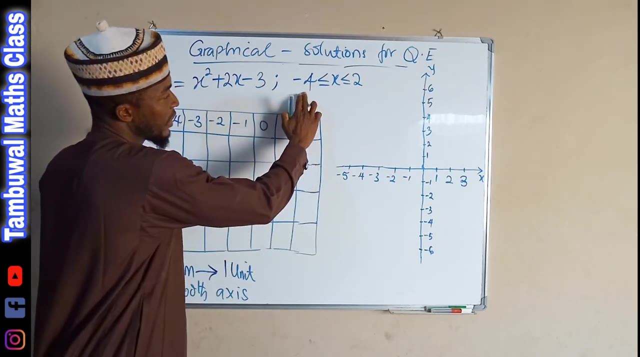 solution for this equation graphically and we are given the range for x values from negative 4 to positive 2, which is going to appear in our table. So this is how to plan your table. The first row are the values of x given to us, from negative 4 to positive 2, and I have already arranged them from negative 4 to positive. 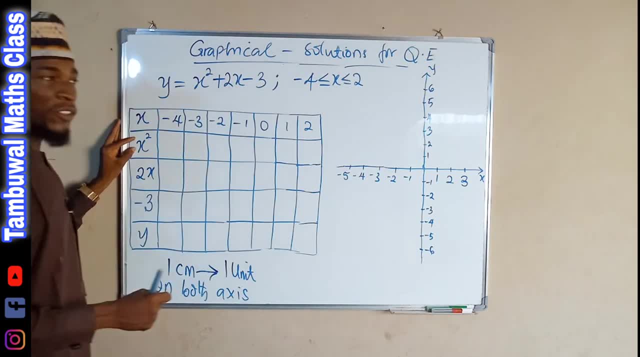 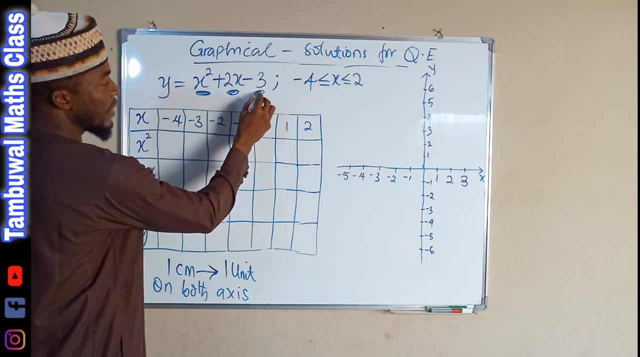 2.. The second row are the values of x squared, and x squared is the first term we have from our equation. The third row are the values of 2x. The fourth row are the constants, which is the last term in our equation, And the last row are the values of y, after simplifying. 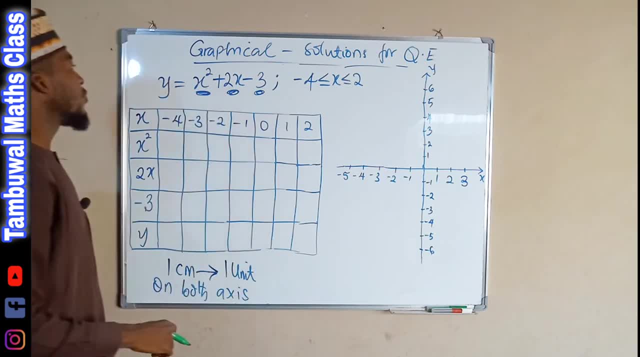 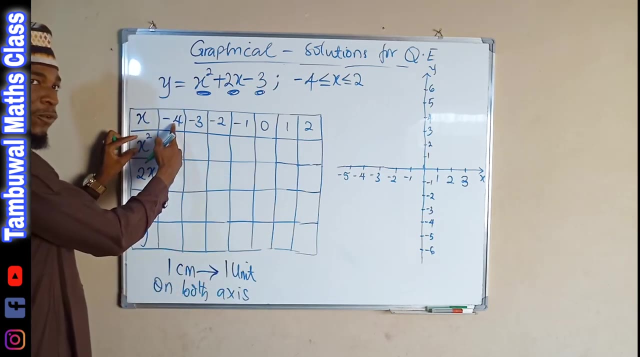 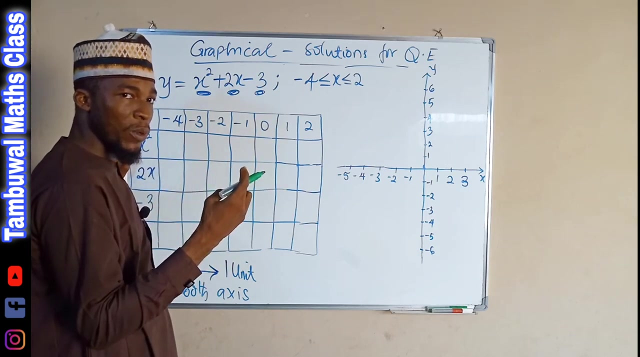 The values of x in the main equation. So what we are going to do after arranging our values in this form, we want to insert the values of x squared here throughout. So we say: when x is negative 4, what is negative 4 squared? Negative 4 squared meaning negative 4 times negative 4, which is: 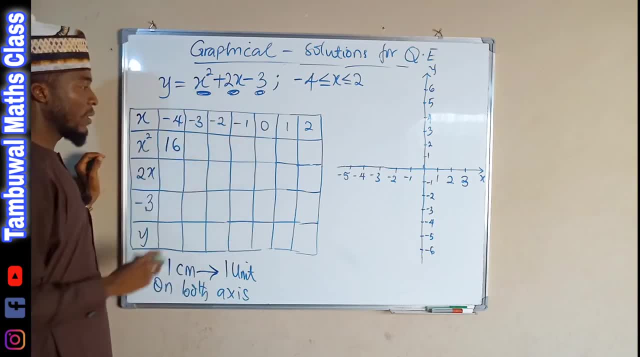 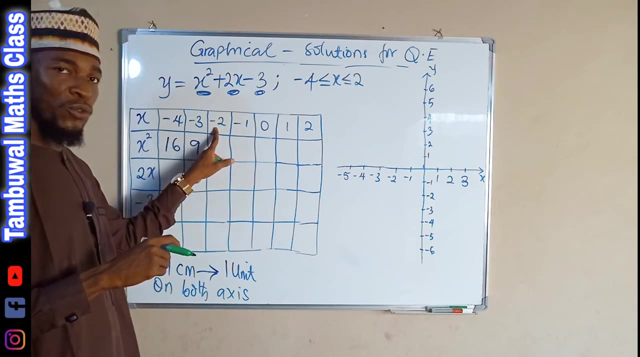 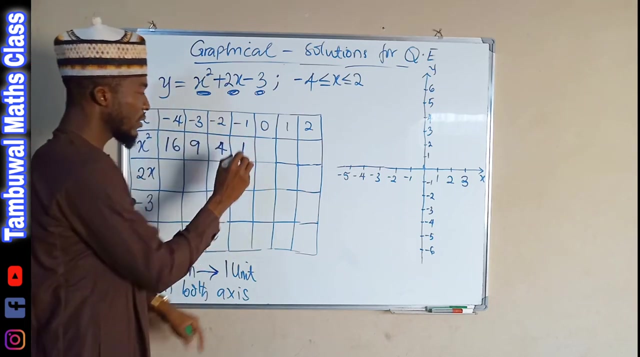 positive 16.. Here we have x to be equal to negative 3, and what is negative 3 squared, It's negative 3 times negative 3, which is positive 9.. We have negative 2 squared positive 4, negative 1 squared positive 1, zero squared is zero. 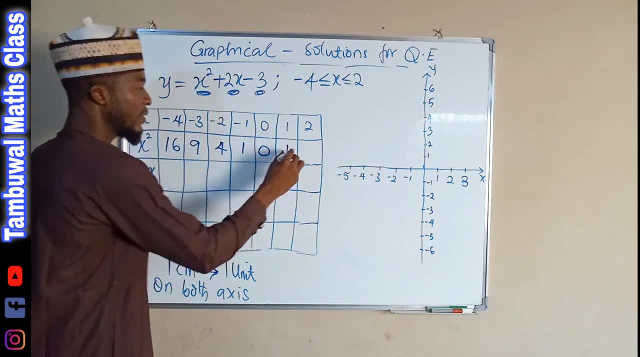 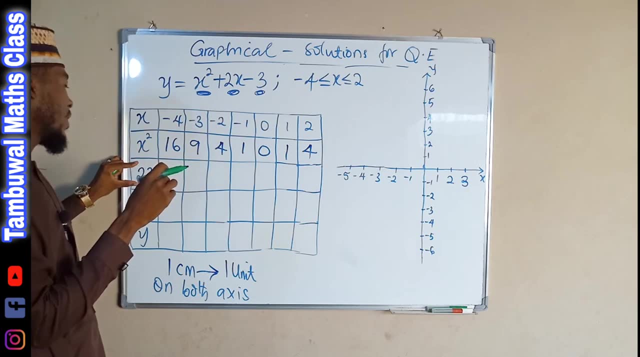 1 squared is 1,, 2 squared is 4.. Then we move to 2x, which is the middle term. We substitute the values of x in that term, 2 times x, meaning 2 times negative 4, and we have negative 8.. 2 times x, 2 times negative 3, we have negative 6.. 2 times x. 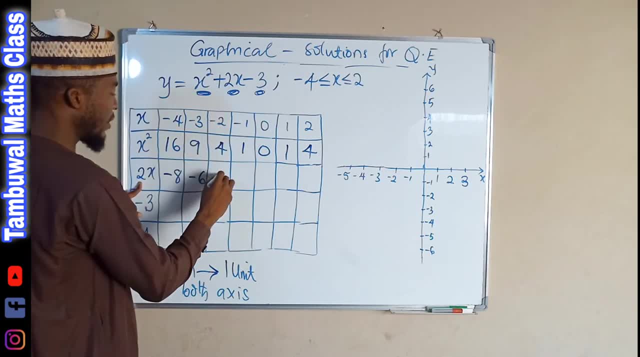 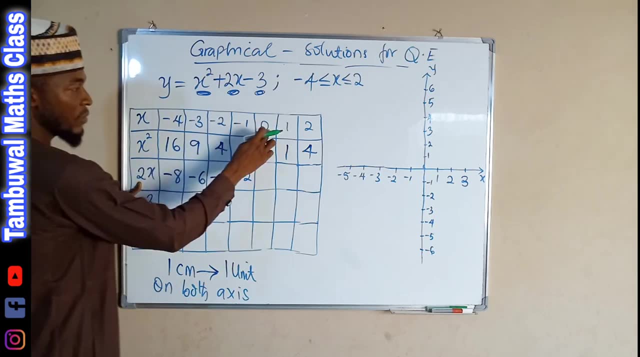 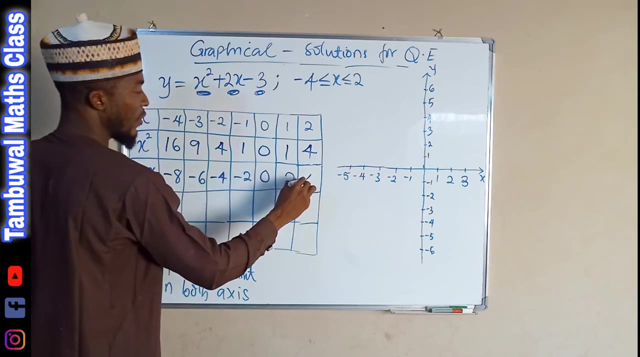 2 times negative: 2, we have negative 4.. 2 times negative: 1, we have negative 2.. 2 times 0, we have 0.. 2 times 1, we have 2.. 2 times 2, we have 4.. Negative 3 is constant. therefore. 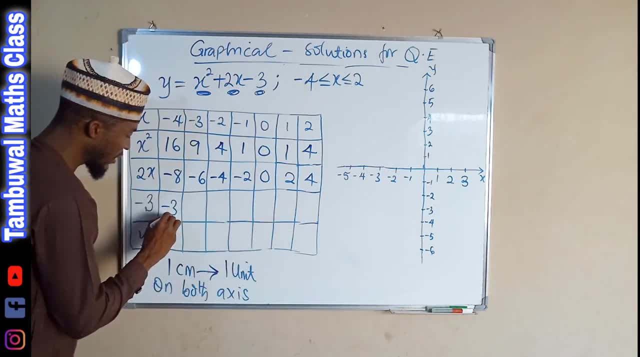 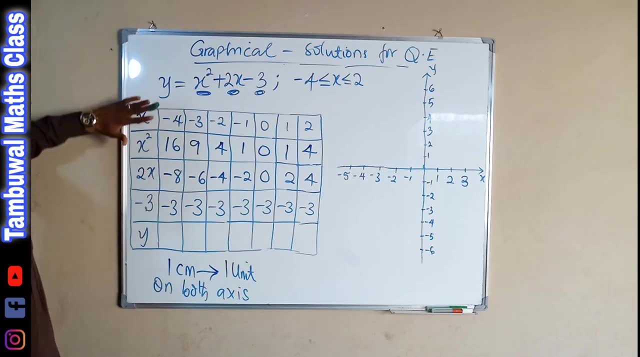 we are going to repeat it throughout. So we have negative 3.. So how do we obtain the value of y? To obtain the value of y, do not consider the first row. We are going to compute these three rows to determine the value of y. So we say: 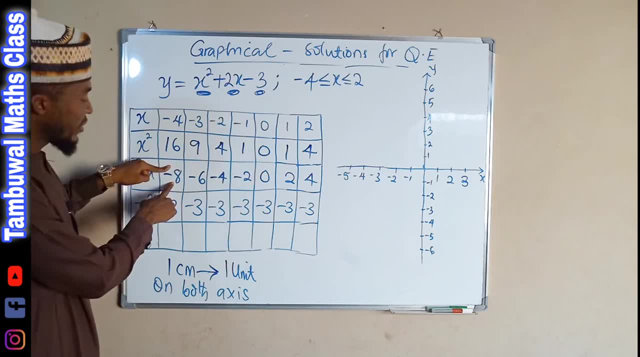 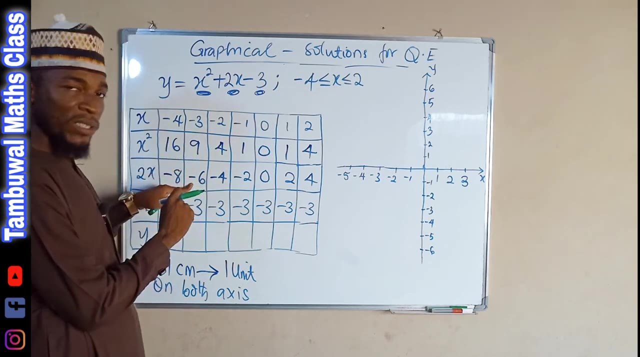 16 minus 8 is positive 8. Then 8 minus 3 is positive 5. So we have 5 as the value of y. Then we say 9 minus 6 is positive 3. Positive 3 minus 3 is 0. Then we move to the next one. 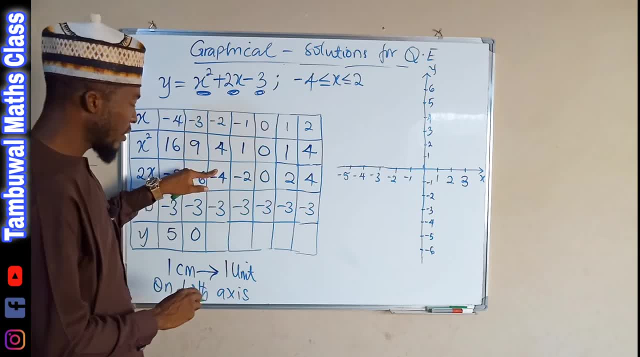 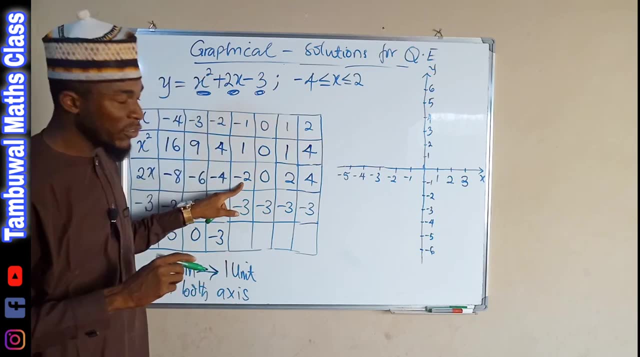 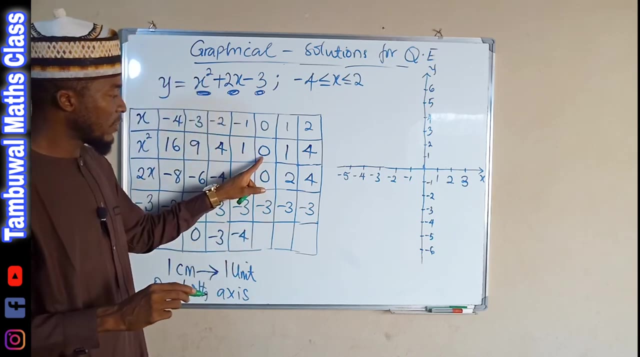 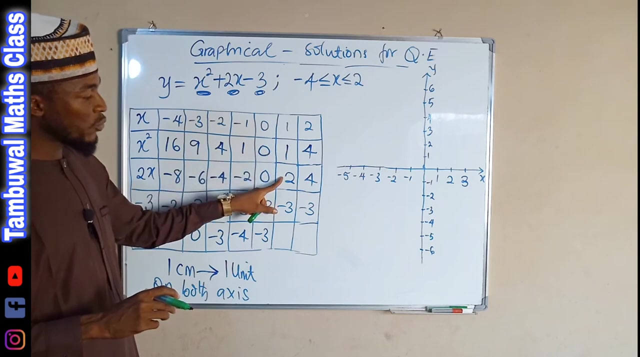 4 minus 4 is 0.. Then 0 plus negative 3 is negative 3.. 1 minus 2 is minus 1.. Then minus 1 minus 3 is minus 4.. 0 plus 0 is 0.. Then 0 plus negative 3 is negative 3.. Then 1 plus 2 is 3.. Then 3 minus 3 is 0. 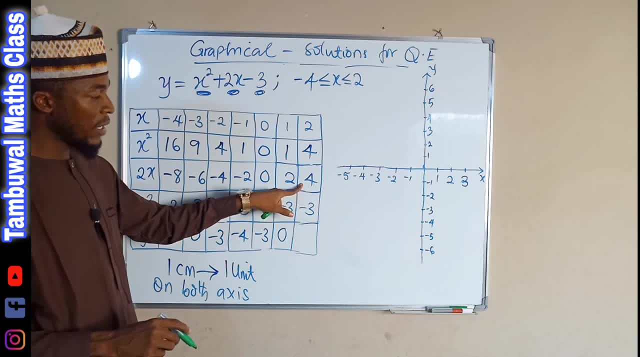 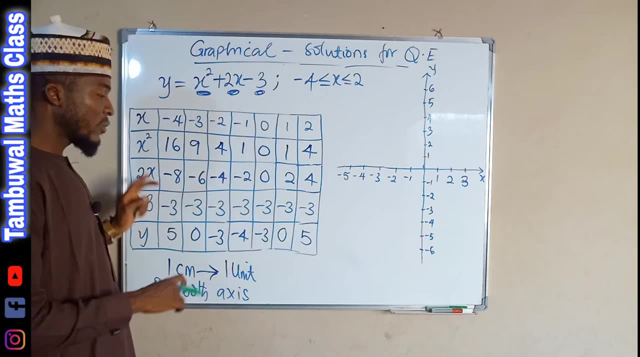 Then we have: 4 plus 4 is 8.. eight, then eight minus three is positive five. So now we have finished computing our table and we are given scale as one centimeter to represent one unit on both axis, and already we have our y and x axis. 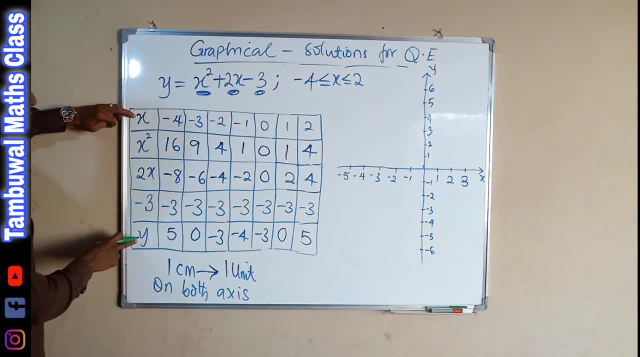 We are going to construct this graph of x against y. So let's begin When x is negative four. we have the value of y to be equal to positive five. So we are going to locate negative four on x axis, then we locate positive five on y axis. 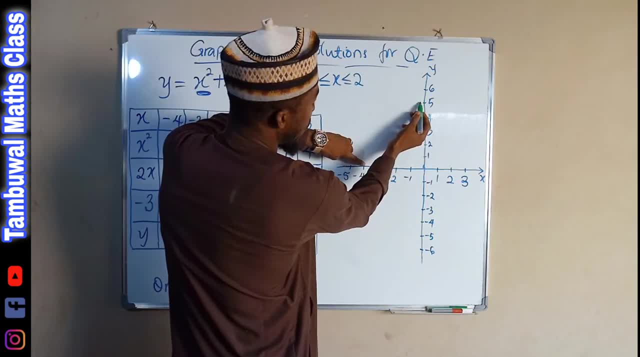 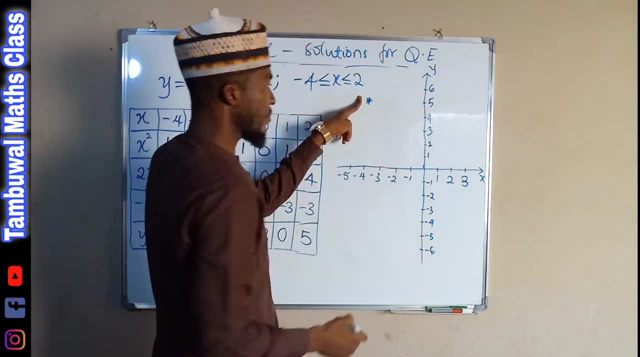 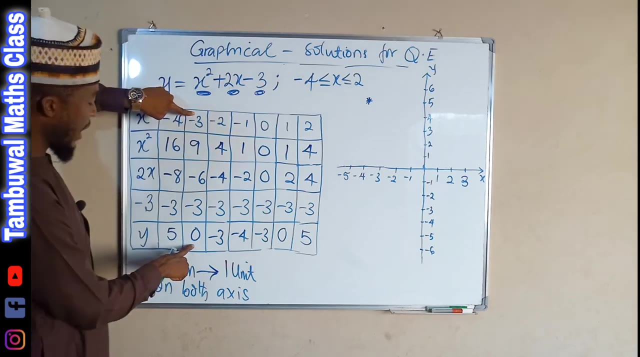 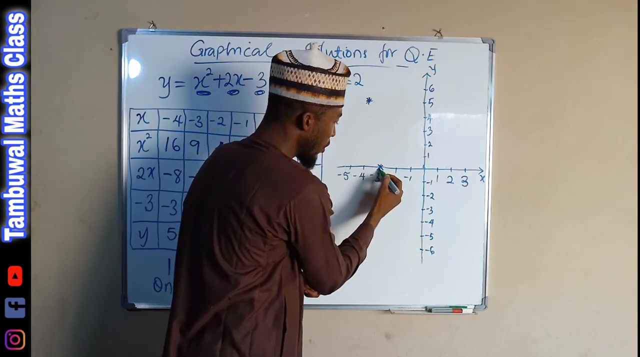 We have negative four on x axis and this is positive y on y axis. the point of intersection, we mark it as asterisk. Then when x is negative three, We have y to be equal to zero. When x is negative three, y is zero. so we mark on the axis. 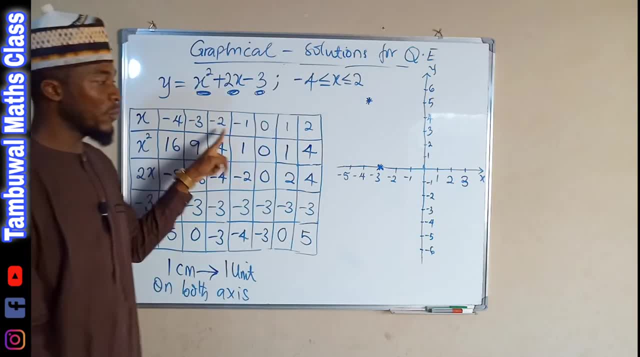 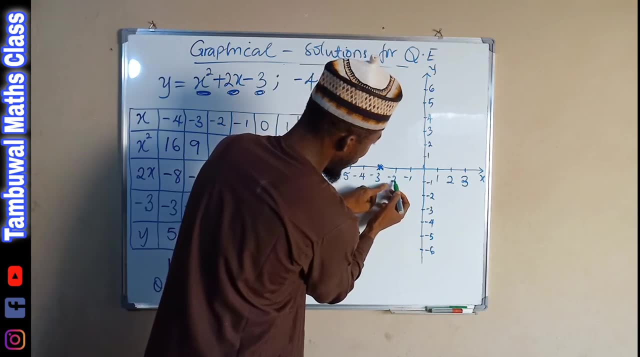 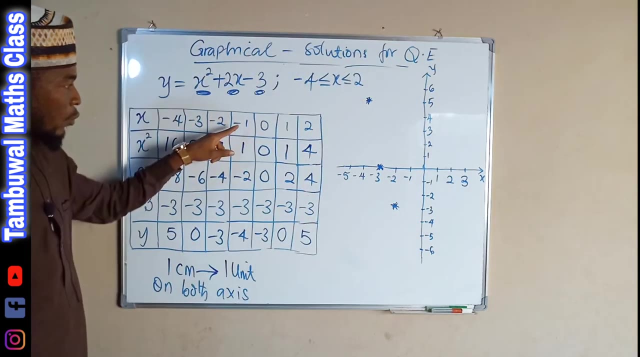 There we move again. When x is negative two, this is negative two for x. We learnt that x is negative three. Negative two, negative three. this is the intersection between them. We mark it as asterisk. When x is negative three, y is zero. 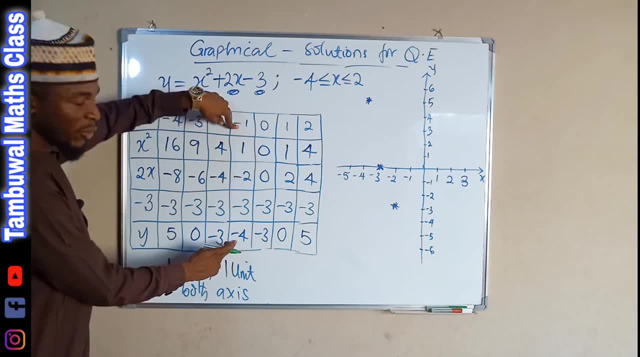 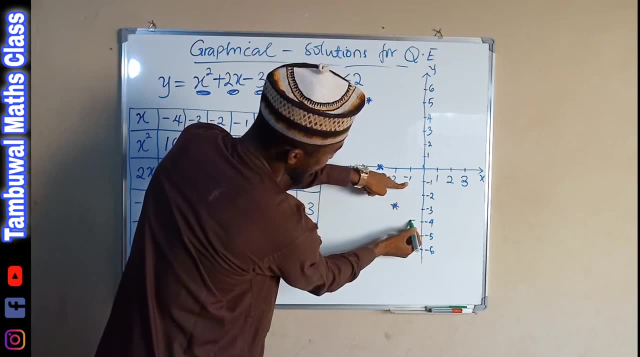 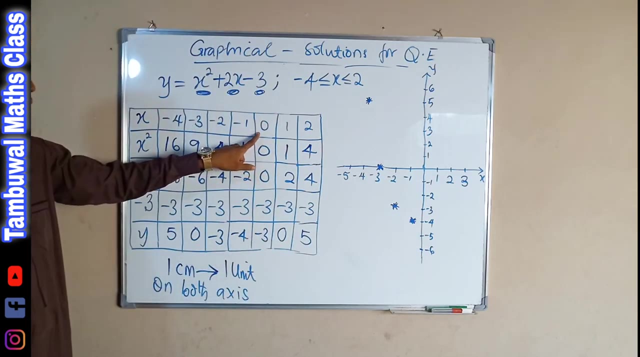 When x is negative one, we have the value of y to be equal to negative four. When x is negative one, we have x to be negative four. so we mark this point, Then we move on. When x is zero, we have y to be equal to negative three. 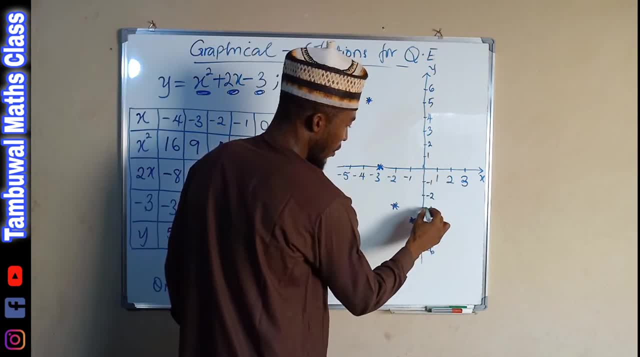 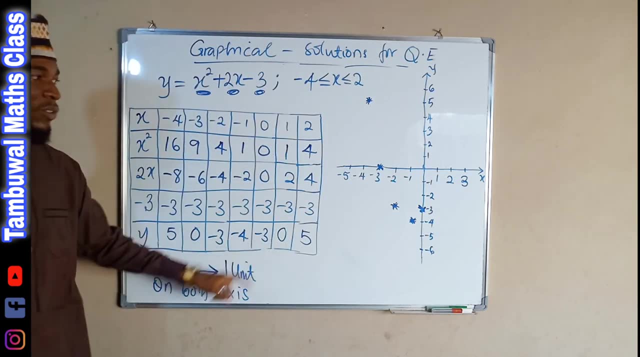 When x is zero, y is negative. three. When x is negative three, y is zero. When x is negative three, y is negative. four. When x is negative three, y is negative. four. When x is negative three, y is negative four. 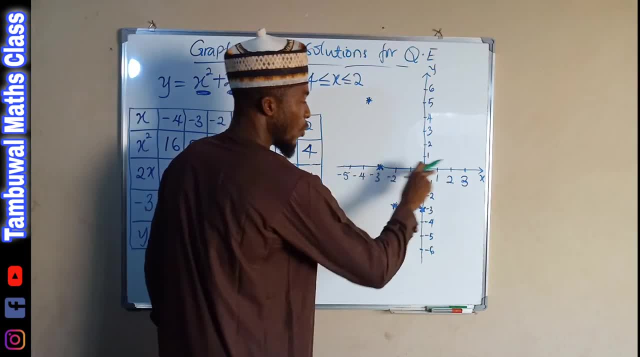 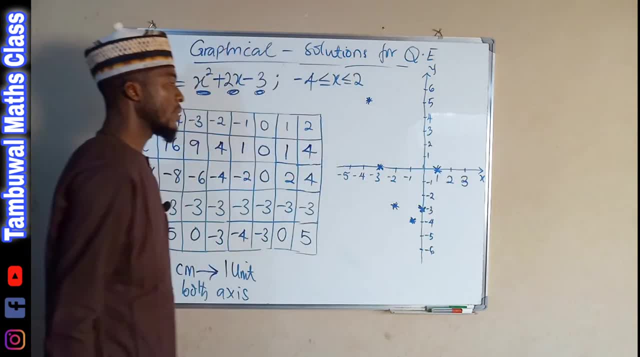 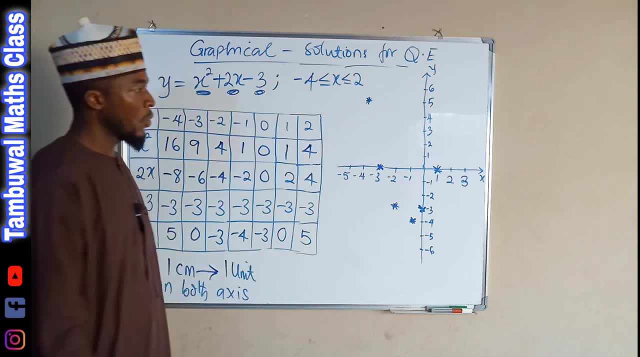 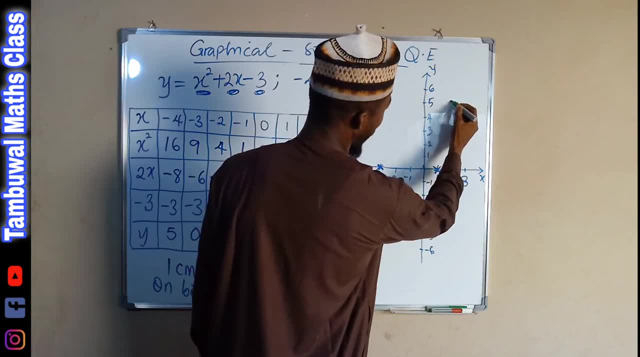 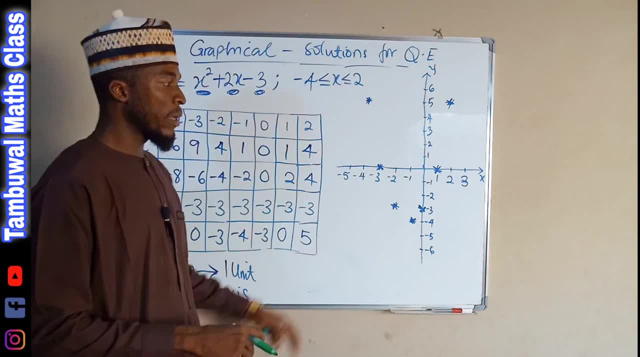 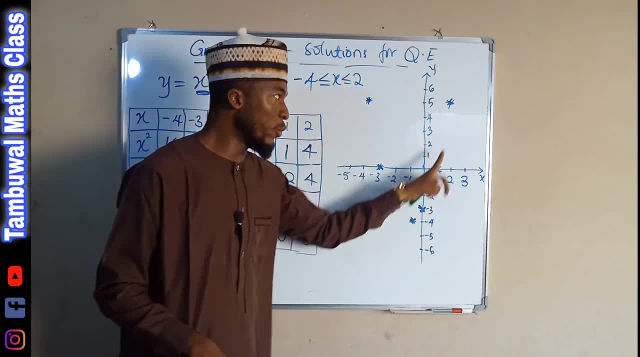 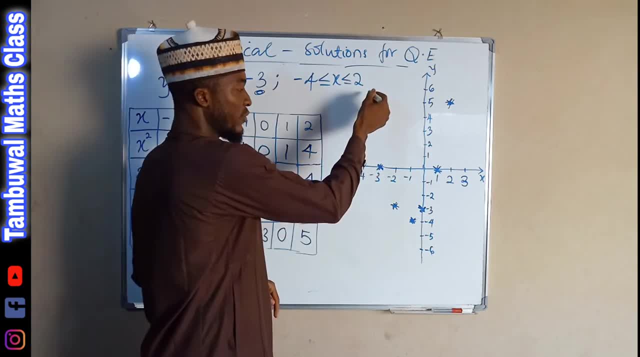 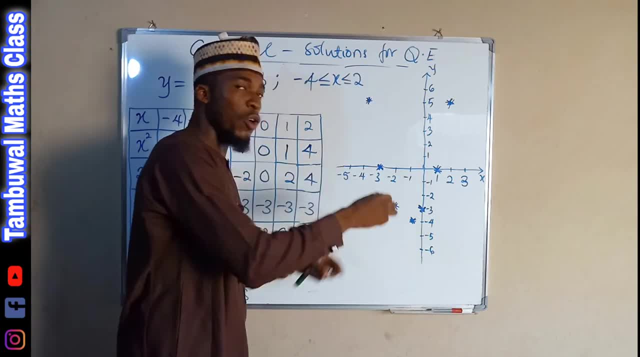 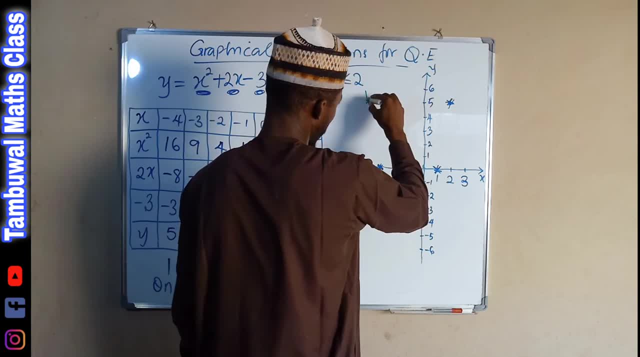 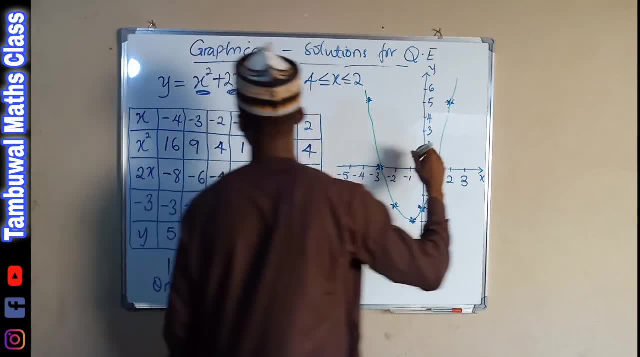 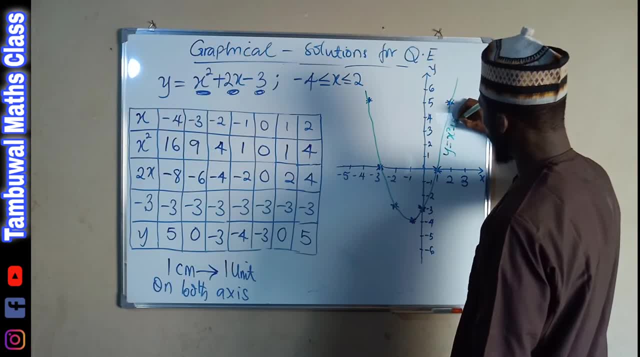 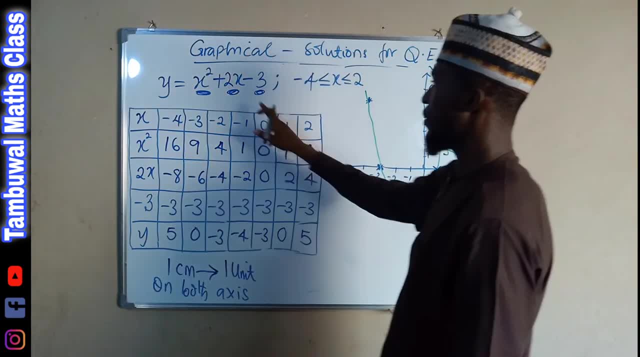 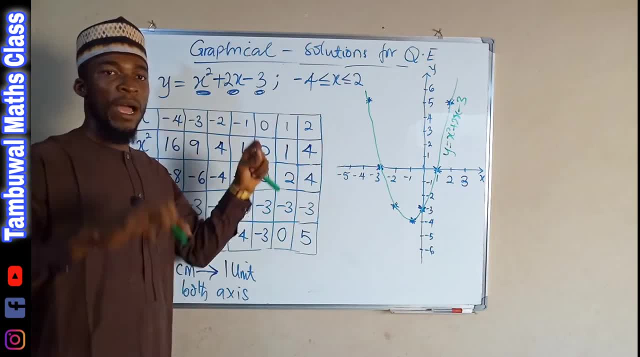 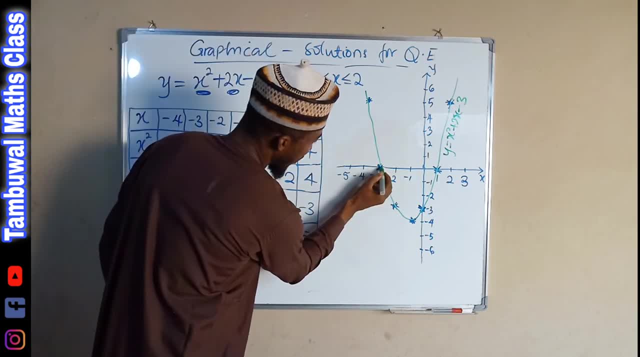 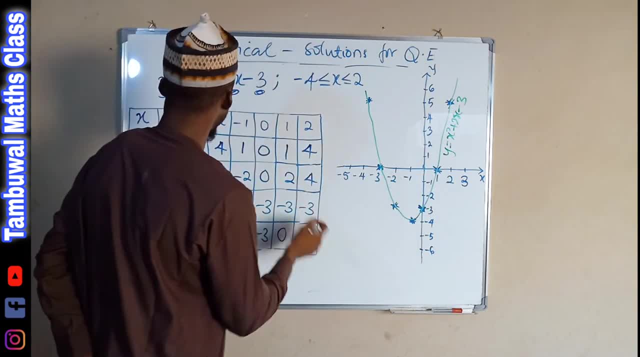 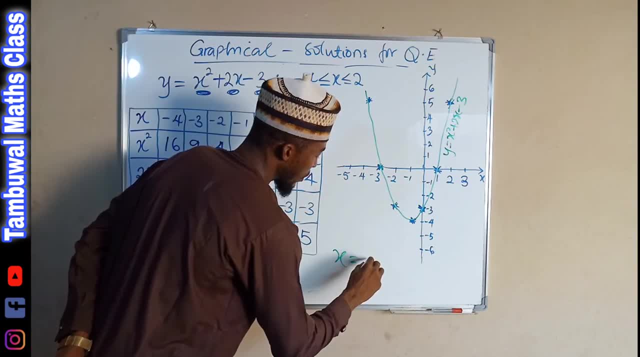 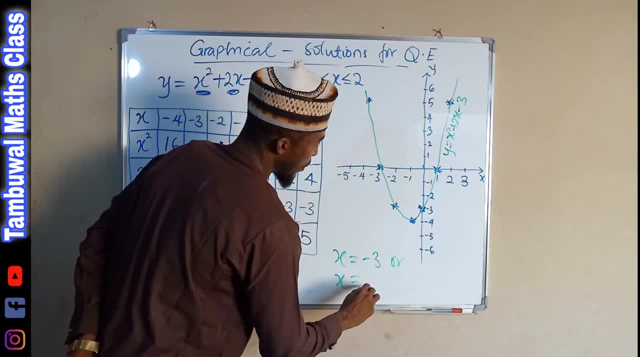 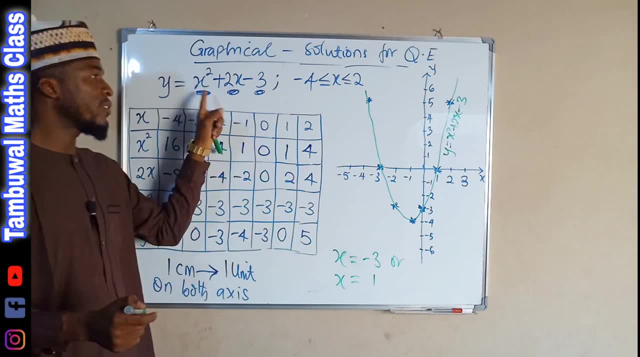